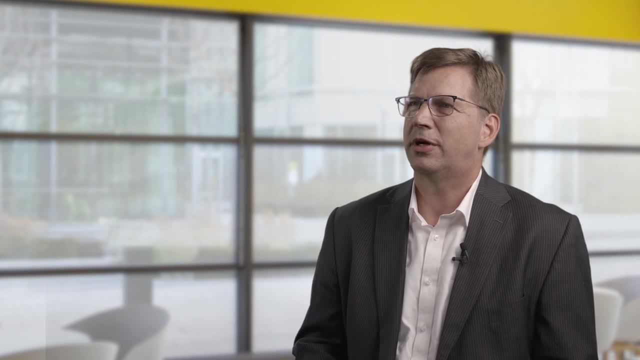 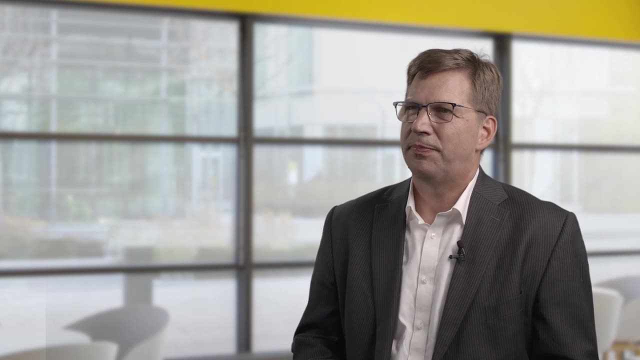 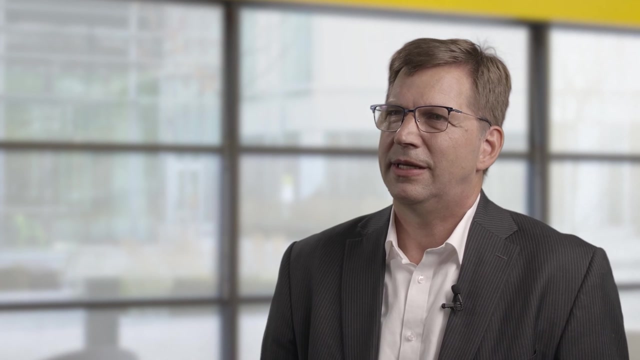 So sound scientific expertise- knowing your product- is critical to taking away the fear of change. Having data available and having guidelines that support our customers to implement process intensification are critical, Obviously, if they have a good molecule and they know the properties of this molecule. 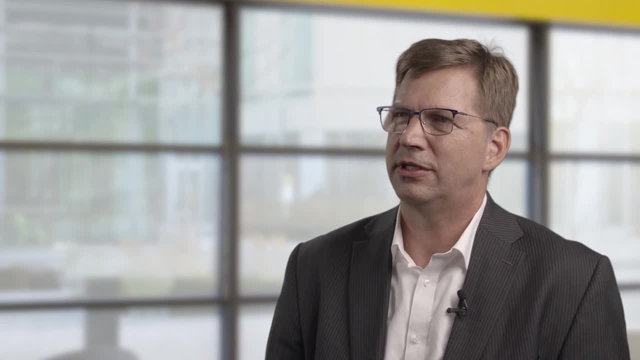 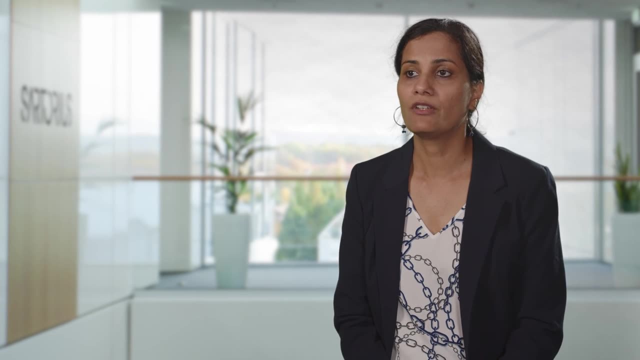 like how productive the cell line is and how stable the product is. they can use this knowledge to implement the process. intensification approaches: Having the right tools, for example, having the right PAT tools or the automation tools to manage the risks. What is the fear of change? 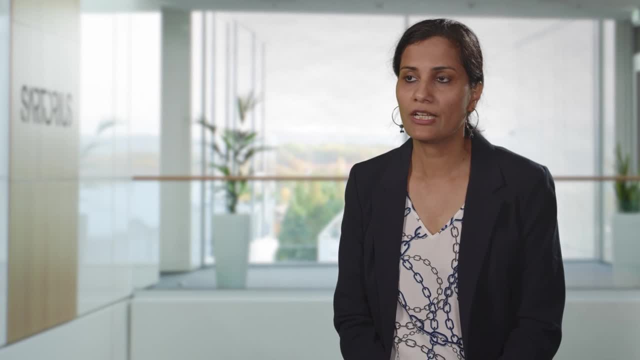 The fear of change is a risk. to understand your process is very important. All that this would help to you is to reach time to market much faster. So don't be afraid of the change Once a scientific expertise is there, once the technology is there, once you know that. 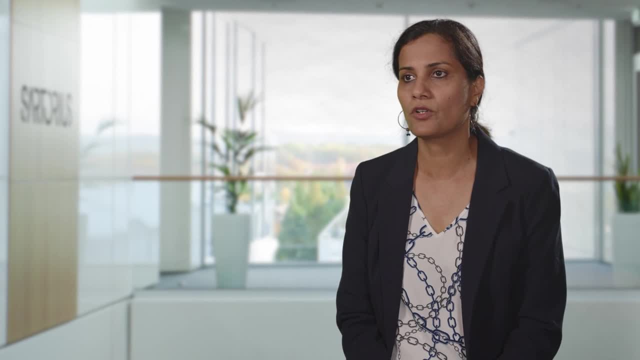 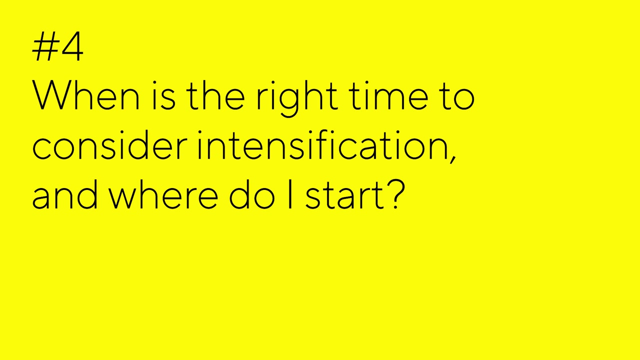 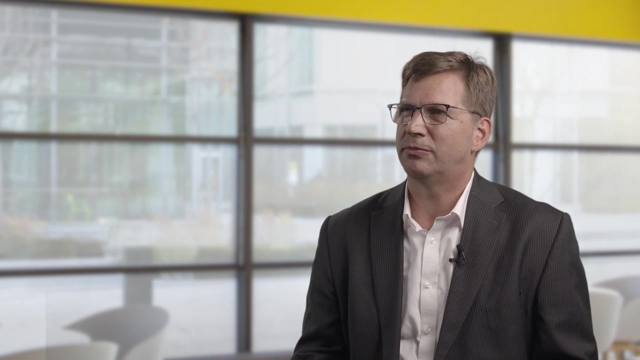 your goals. you can really apply those and do your process development and get the benefits of process intensification, which is higher productivity, lower cost of good and faster time to market. It's critical to start early in process development with your process intensification. approaches. Ideally, you already start with it during your cell line development. Obviously, you also have to consider the further downstream ramifications. In upstream, you can start selecting clones that are high yielding in perfusion conditions, And perfusion is typically the way to intensify your cell line. 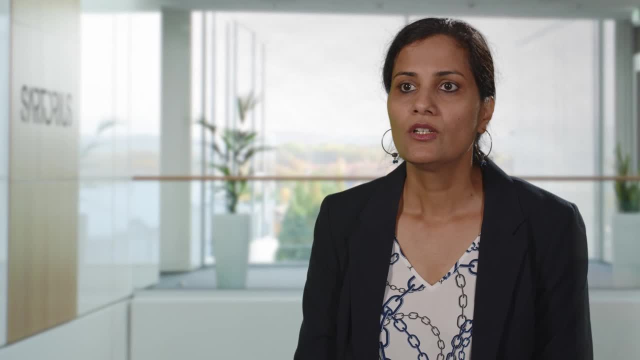 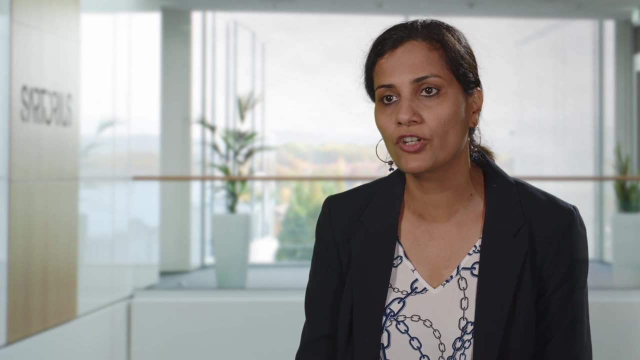 It's important to start early in process development with your process intensification approaches. Ideally, you already start with it during your cell line development, Begin your upstream process. So, knowing your process, having the baseline, understanding your priorities, your goals. what is the end goal that you're trying to reach for your molecule, for your product? 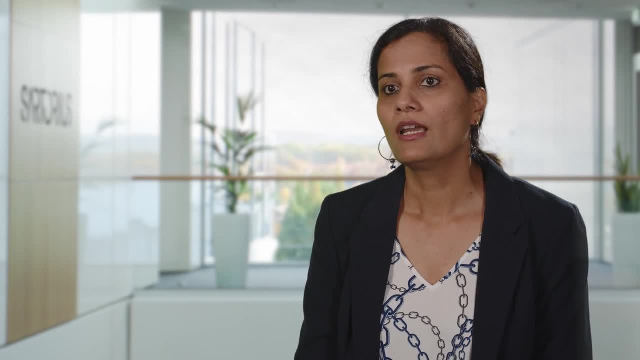 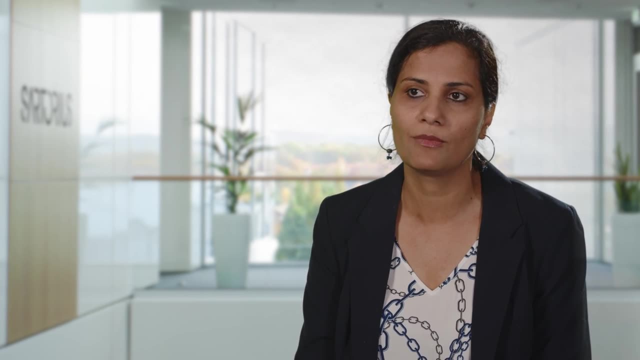 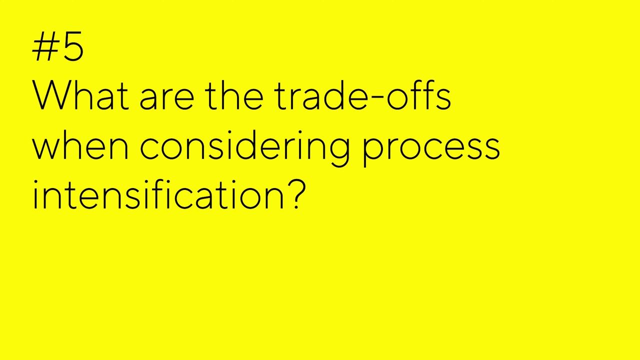 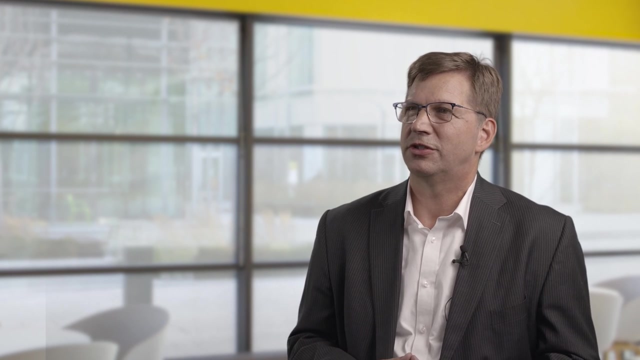 when you go to manufacturing is where you need to start And then apply your process intensification technologies, because there so many different strategies, both upstream and downstream, that you can apply. In general, there are mostly positives for process intensification. What you're. 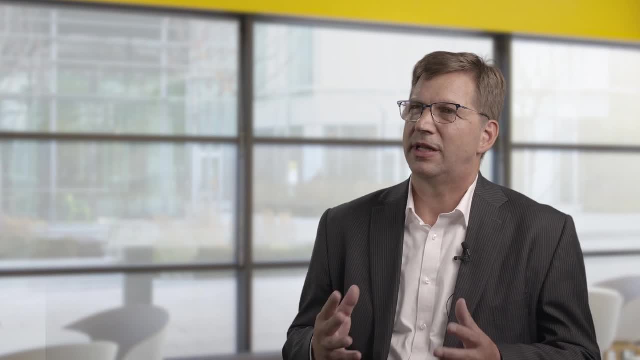 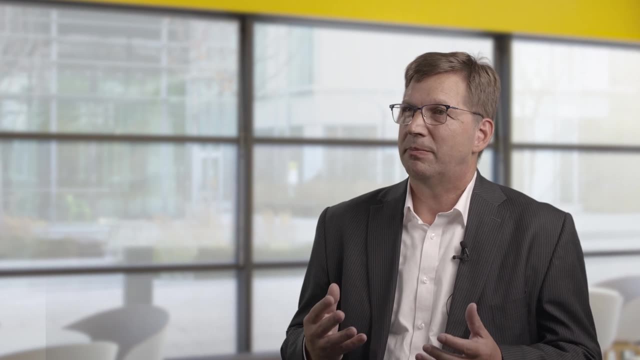 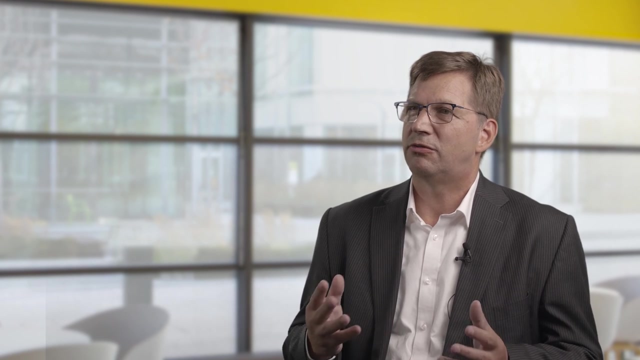 doing is you're increasing the volumetric productivity and this allows you to use smaller process equipment and reduce your facility footprint. And by using smaller equipment, it also allows you to still keep using single-use solutions. This drives down the capital expenditure a lot and allows you to have more cash flow for other projects. Overall, the facility build-up time can also be reduced up to 50%, for example, With smaller facility site which is single-use implementation, you don't really need to build large facilities which can take up to four to five years With implementing process. 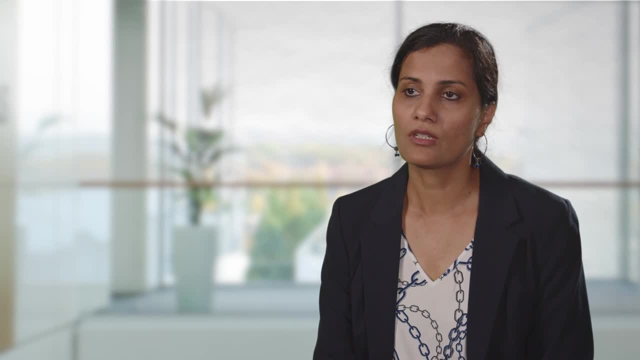 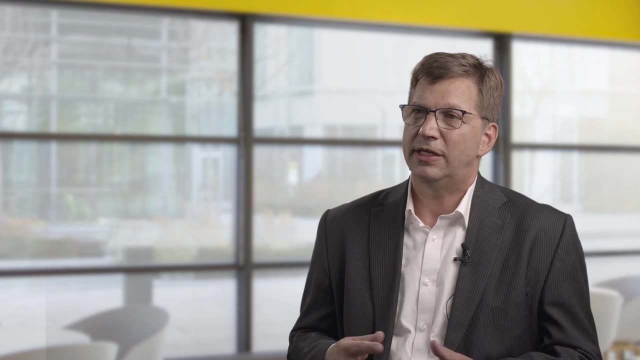 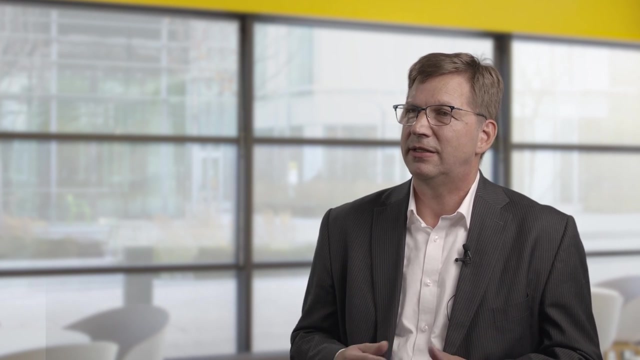 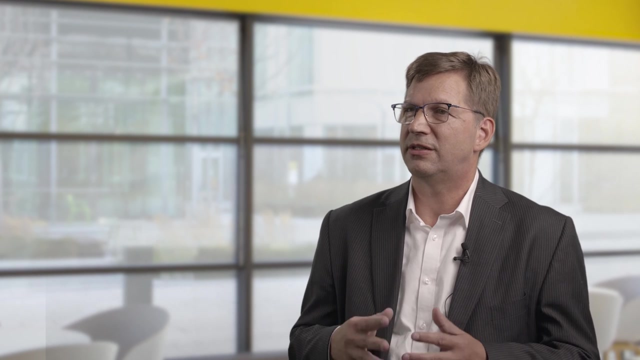 intensification, you can actually build your facility within two years, which really helps time to market your drug and really be the market leader for that drug Trade-off is that the new process approaches need to be developed and validated and this may cost you more time compared to your traditional platform process. Good news, however, is 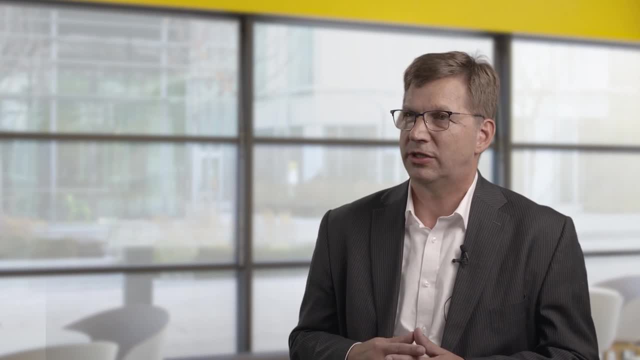 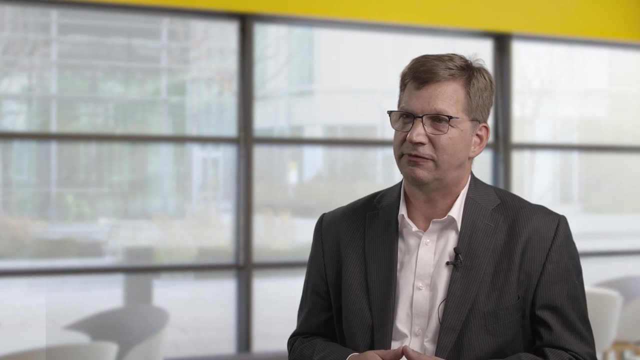 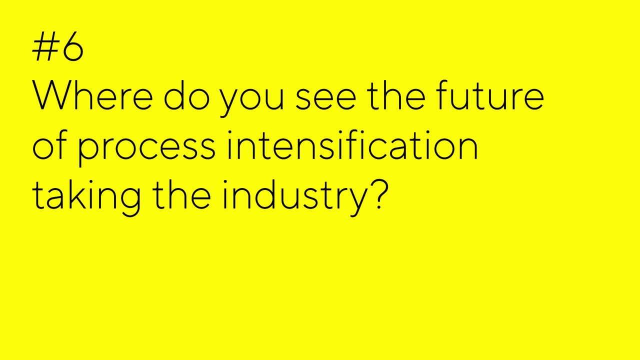 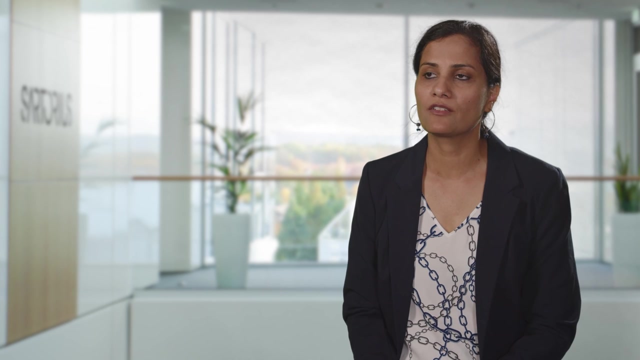 that the right tools are now available to develop these process intensification approaches and they make it easy to implement process intensification- as easy as FEDpatch, As the industry is moving towards bioprocessing 4.0, having highly productive, small and agile facilities which are enabling greater automation. 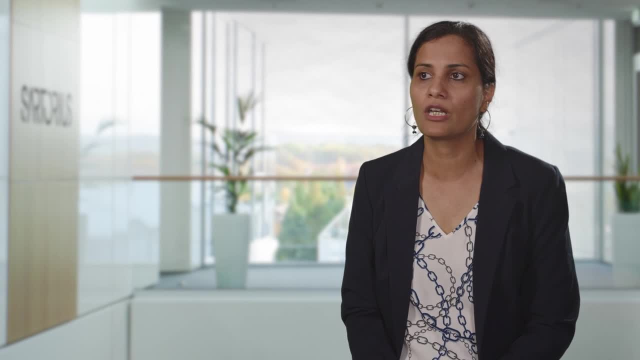 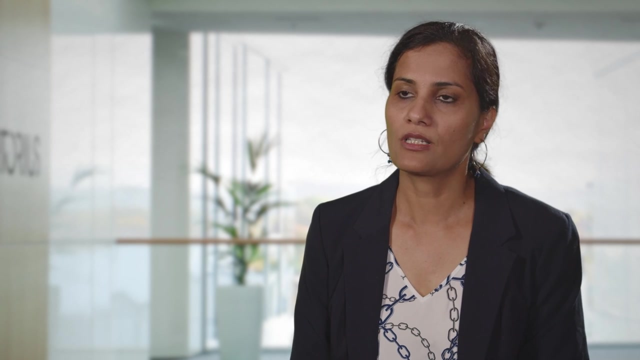 and AI involvement in streaming efficiency through reduction in manual activity is important, So the need of data and the tools to achieve this is going to be very important for anything that people are trying to involve for their future facilities. The other important aspect for process intensification is sustainability. So once you 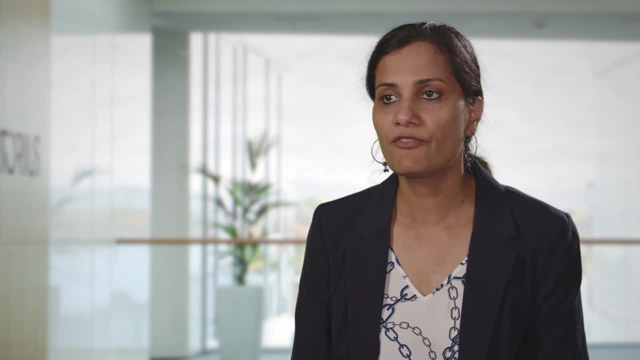 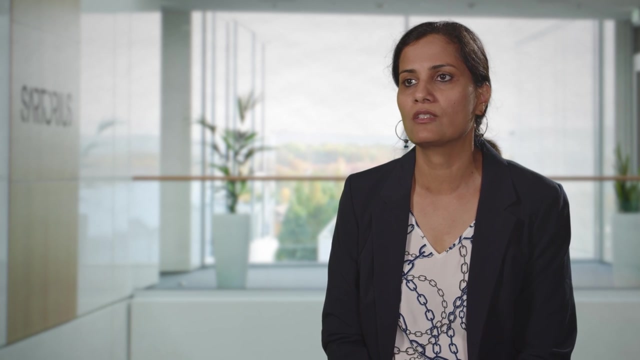 are applying single-use technologies which are in a smaller facility footprint, you would require less amount of water, less amount of energy and also have, hopefully, lesser carbon footprint. So achieving your sustainability goals would become much more simpler and easier. when you apply process intensification, So this data-driven advanced process control option will 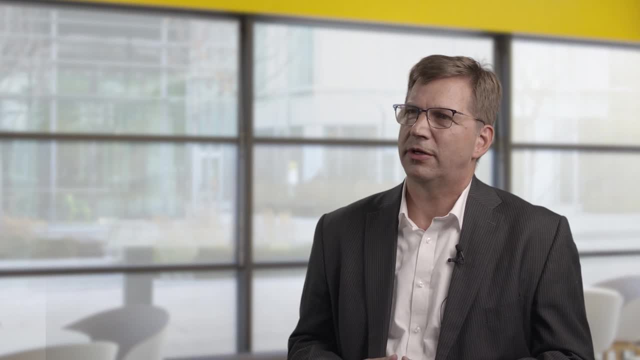 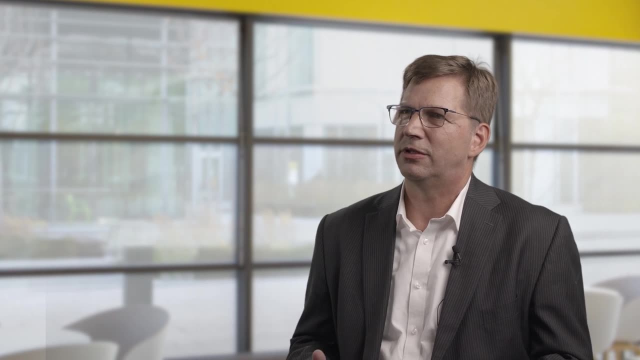 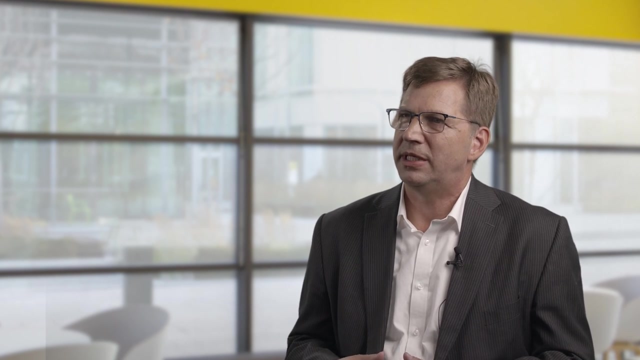 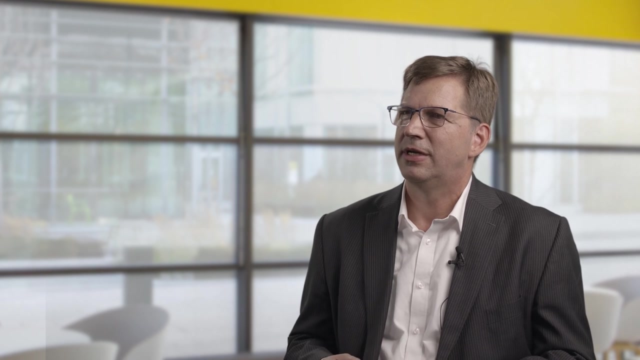 allow us to go to real-time release of our products and drastically improve our process understanding of our highly complex biological processes. And, with bioprocessing 4.0, we will be able to meet the market demand: more flexible, faster, cheaper and better, And especially in these pandemic times, that. 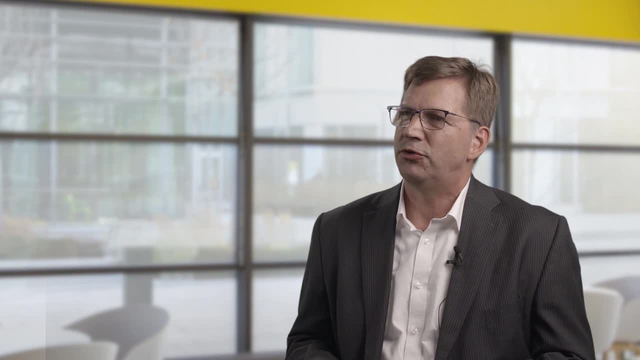 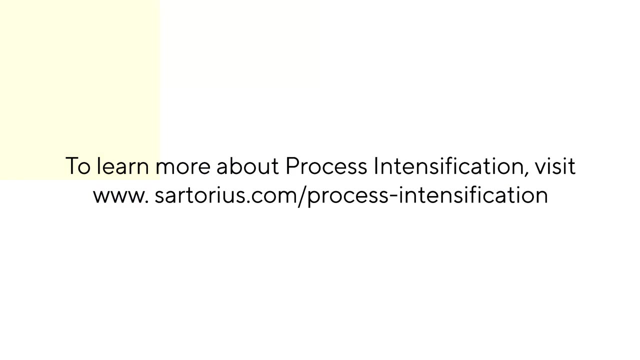 would be, let's say, the ultimate contribution that the biopharmaceutical industry could deliver to solve the issues at hand you